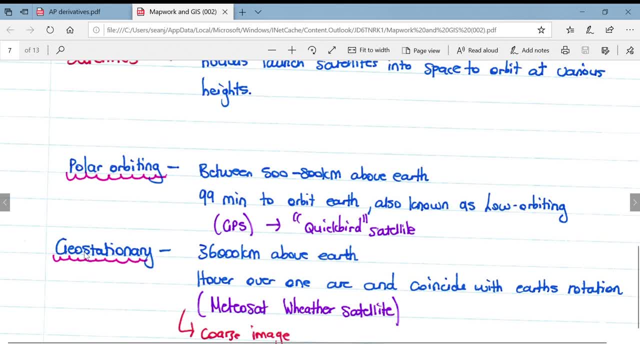 a polar orbiting satellite. then we look at geostationary satellites. these are 36 000 kilometers above the surface of the earth. they hover over one object and are and coincide with earth's rotation. an example of a geostationary satellite image would be the meteorostat weather. 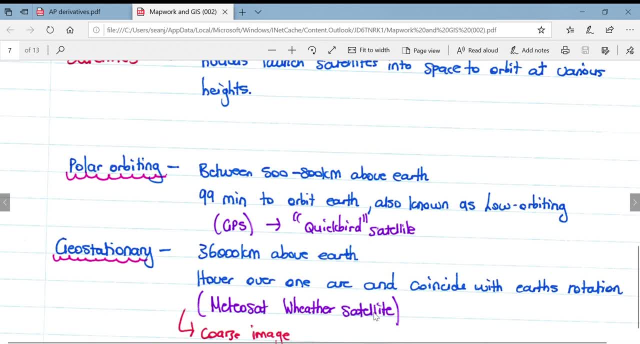 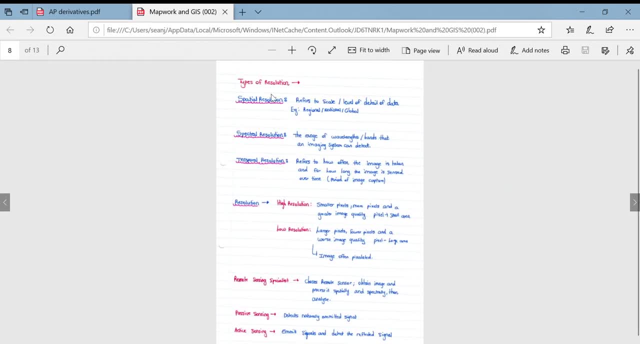 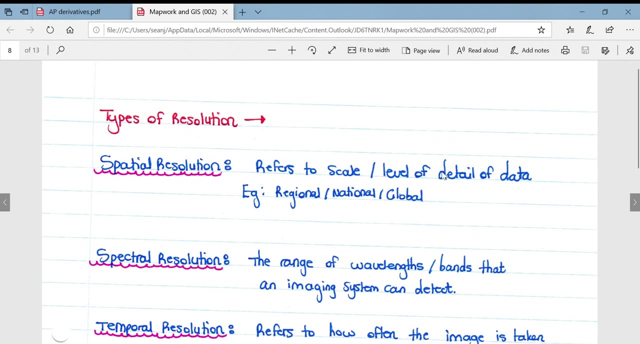 satellite, so a weather satellite image that you see of a whole continent at a time or whatever, and it's often a very coarse image. and if we go on to types of resolution, spatial resolution refers to the scale or level of detail of the data, ie is it regional, national or global spectral. 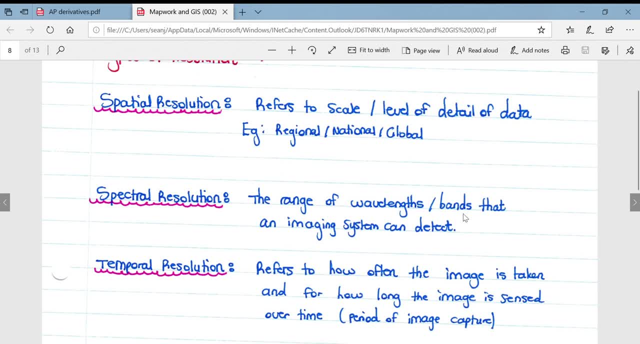 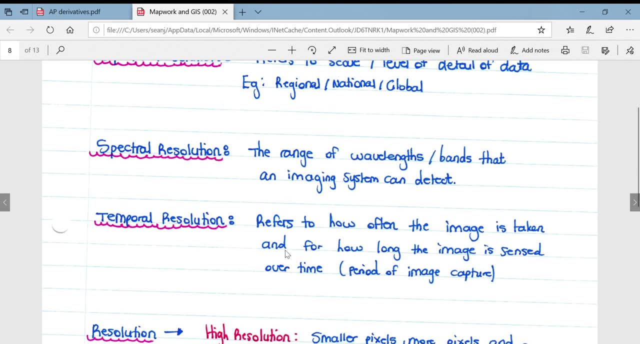 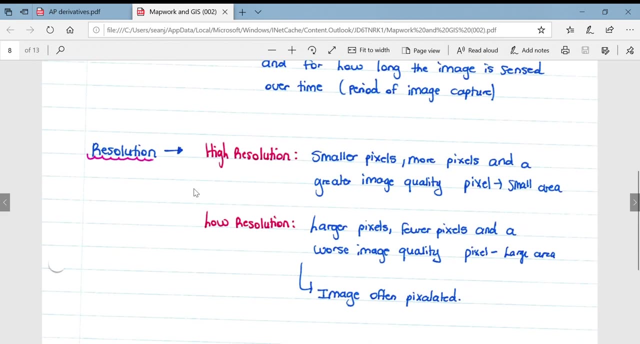 resolution refers to the range of wavelengths or bands that an imaging system can detect. temporal resolution refers to how often the image is taken and for how long the image is sensed over time. it's the period of image capture. then, if we look at resolution, we either get a high resolution, 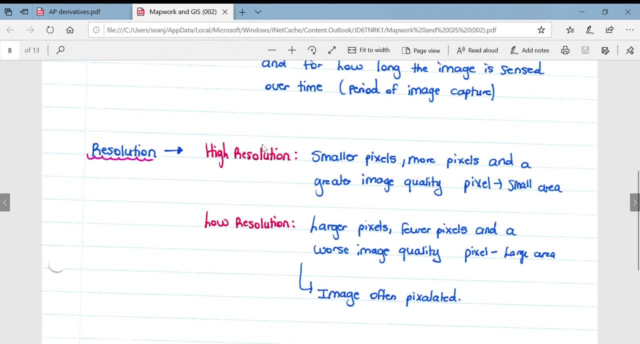 image or a low resolution image very easy to understand. higher resolution image, smaller pixels, more pixels and a greater image quality- the individual pixels cover a smaller area. if we look at a low resolution photograph- larger pixels, fewer pixels and a worse image quality- the pixels often cover a large area. 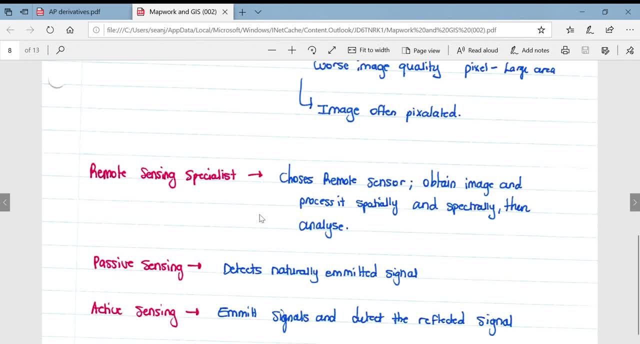 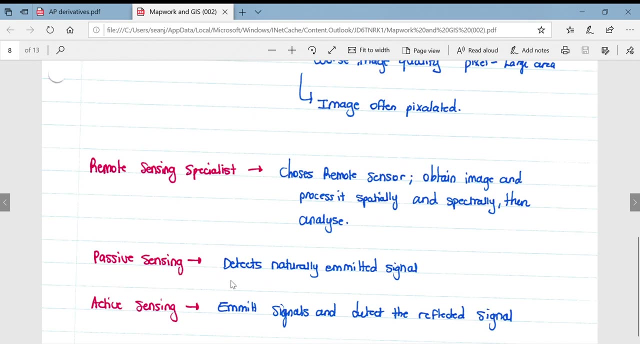 the images often seem to be pixelated. then if we look at a remote sensing specialist, this is a person who uses remote sensing to obtain an image and process it spatially and spectrally, then analyzes the image and sees what it has to tell us. then, if we look at passive sensing, this detects: 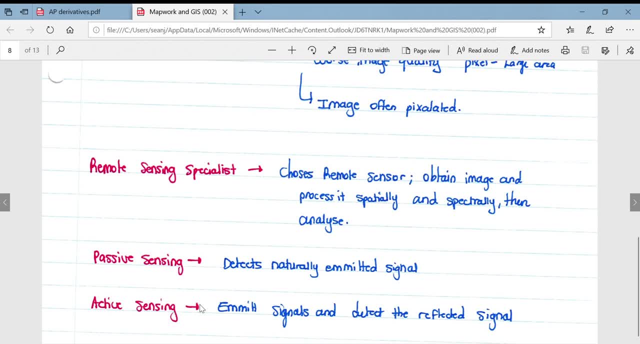 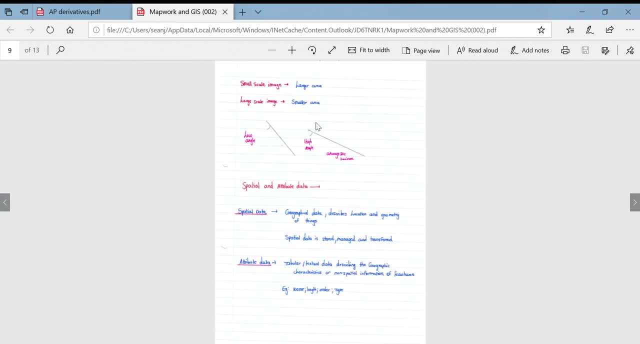 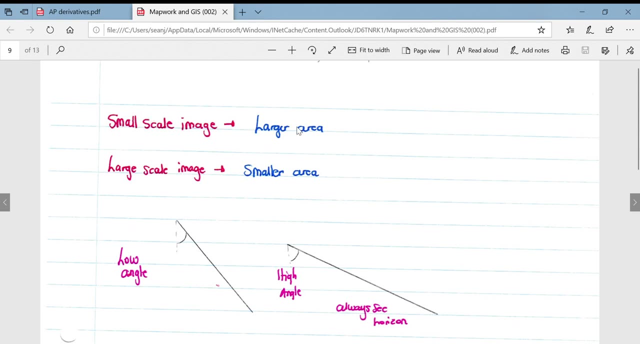 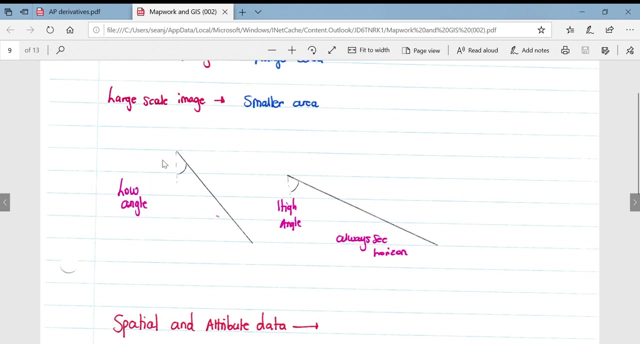 naturally emitted signal. if we look at active sensing, it emits signals and detects the reflected signal of different objects. then if we look at particle violations, image or a affected person or anywhere else we look at a type of image, it can basically detect a variableware or or an object we just için at saja. 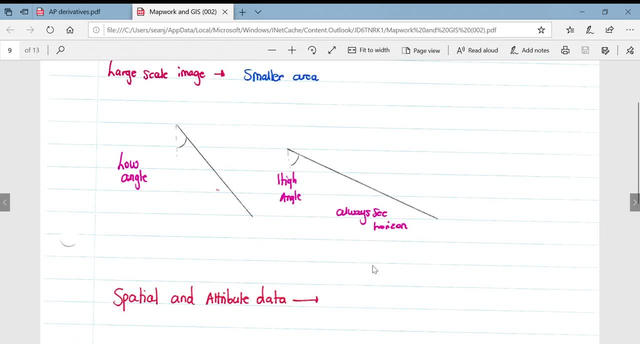 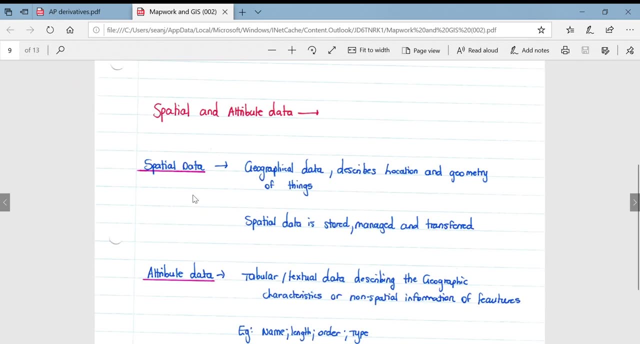 so you can get a taste for most of the images here: small scale and large scale images. obviously, a small scale image covers a larger area, whereas a you can always see the horizon. Then if we look at spatial and attribute data, please note this is one of the most important parts of GIS and one of the areas where they like to test on Spatial data. 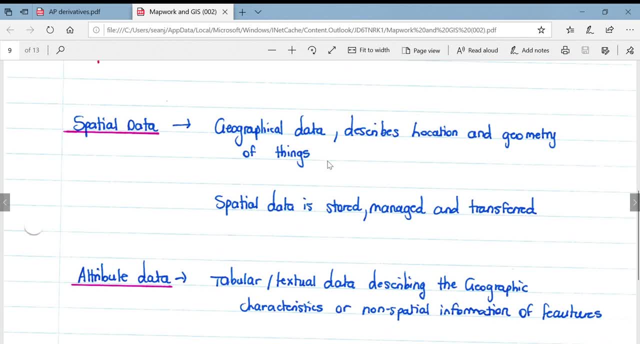 is geographical data, which describes the location and geometry of certain objects. Spatial data is stored, managed and transferred, So an example of this would be the actual base map that you use. So in GIS, open street map is an example of spatial data. It is the background map that you 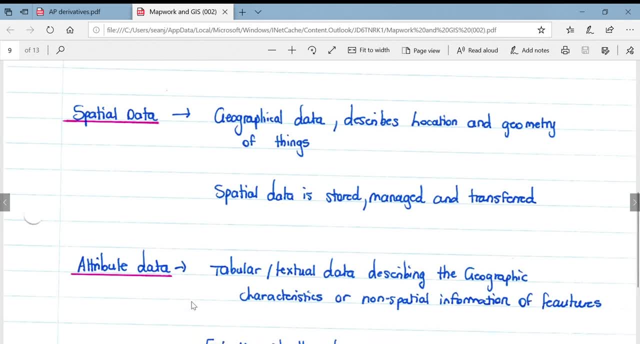 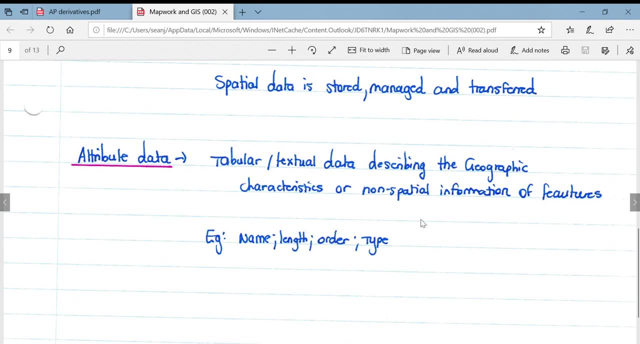 use before you go and input your attribute data. Then, moving on to attribute data, this is tabular or textual data which describes geographical characteristics or non-spatial information of certain features, ie the names of features, lengths of features, lengths of rivers maybe. 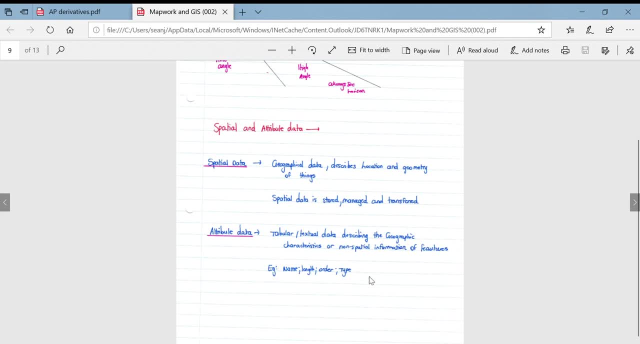 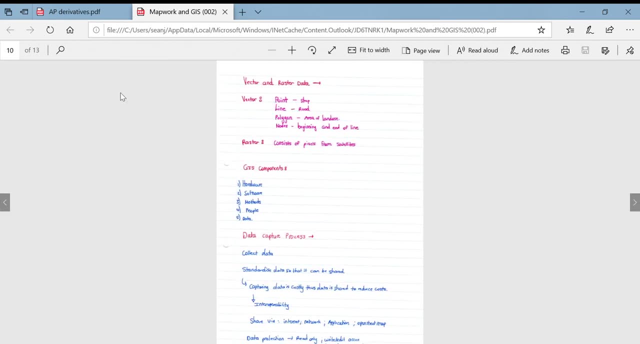 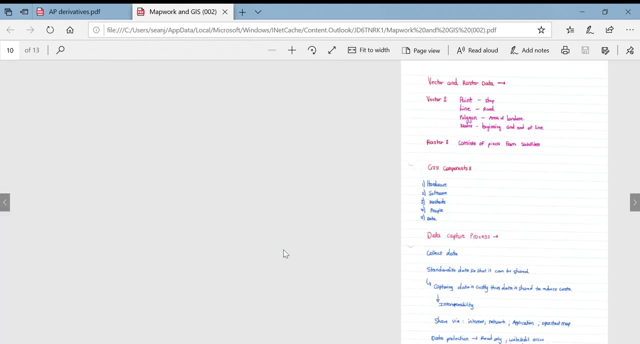 the order of features and the type of features. So you know, like categorization etc. categorizing them into rivers or dams or oceans, etc. Then, if we look at vector and raster data, this follows on from our spatial and attribute data. 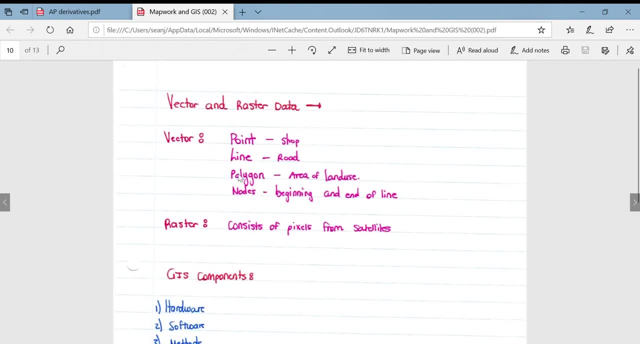 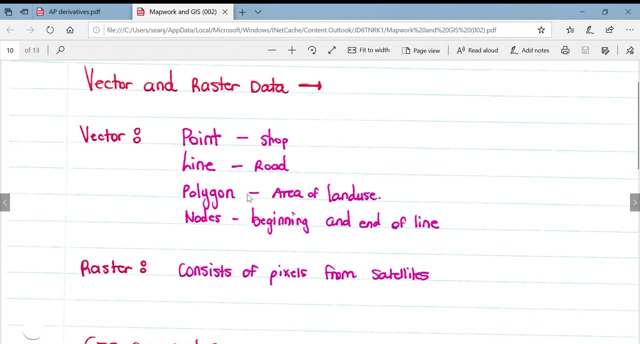 Vector and raster data. vector data comprises of various different representations. We get points, lines, polygons and nodes. An example of point data would be a shop shown on a map- Aligned data and a polygon would be a road shown on a map. Polygon would be an area of land use, such as a farm. 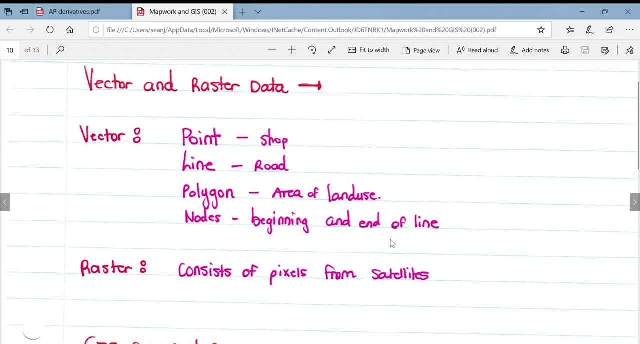 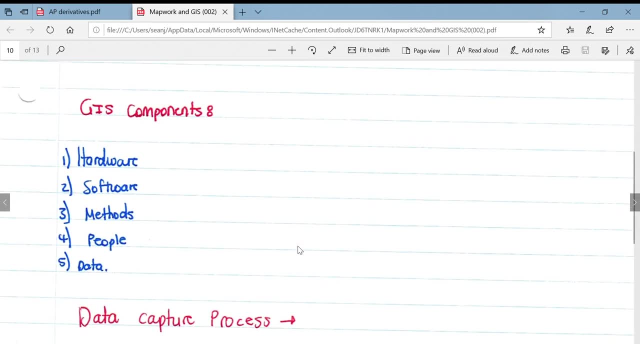 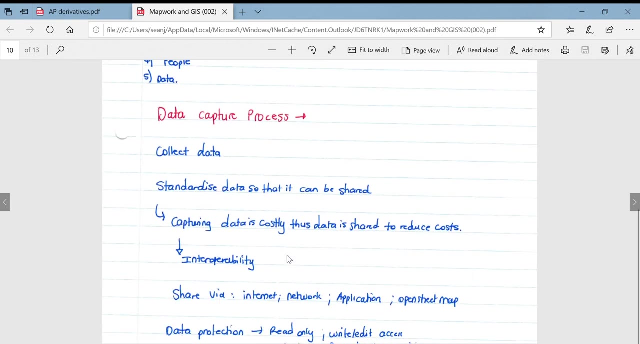 Nodes are the beginning and end of line data. Then, if we look at raster data, this consists of pixels from satellites, The GIS components, hardware, software methods, people and data Data capture process used by GIS. Firstly, collect the data, standardize the data so that it can. 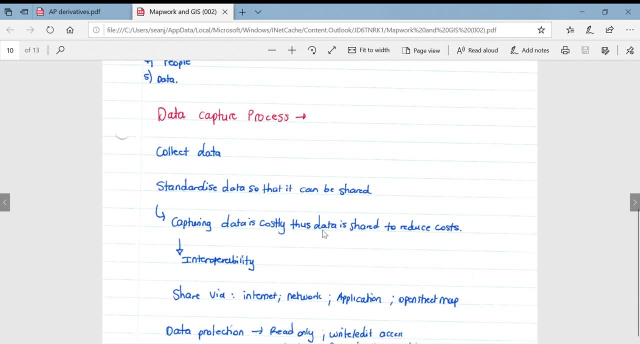 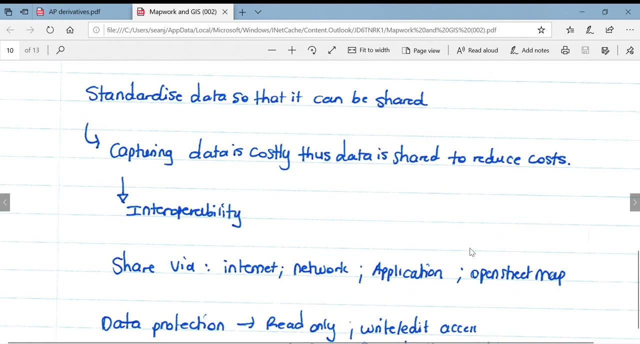 be shared. Capturing the data is costly. thus data is shared, Such as a Roman model, But if you want data, you can use a�를 to do so- reduce costs, which then leads to interoperability. we can either share it by the internet network application or open street map. open street map is: 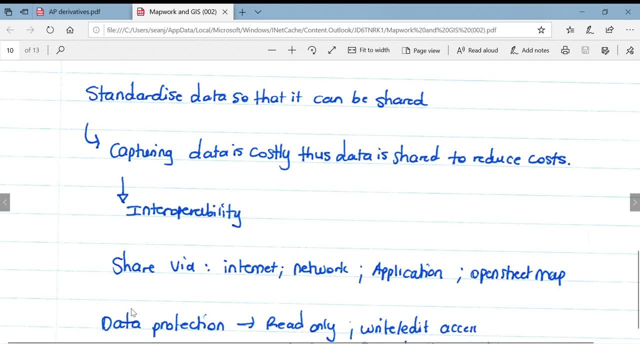 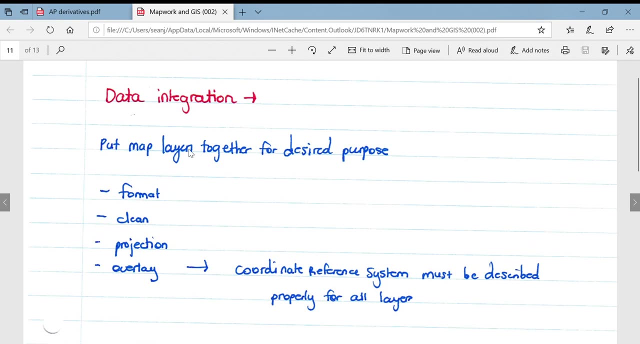 obviously the most common base map used in GIS. then if we look at data protection, often this data is shared as read-only data. I, either people that receive it, cannot write or edit the data. then if we look at data integration, this is where we put multiple layers of a map produced in GIS together and combine. 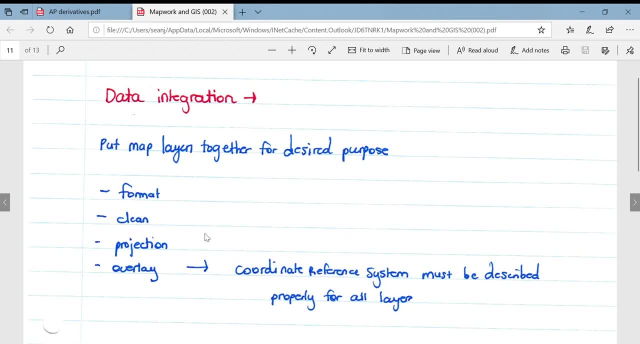 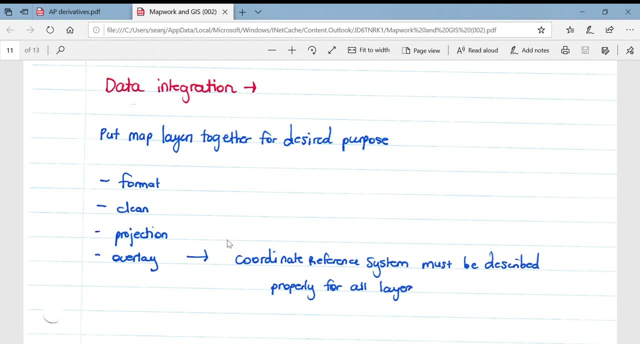 them for a desired purpose and basically what this comprises of is you'll have your open street map, which forms your base map. then you'll also turn on your river layers, your road layers, your main town layers, and all of these combined is known as data integration. so you integrating all of the layers together. 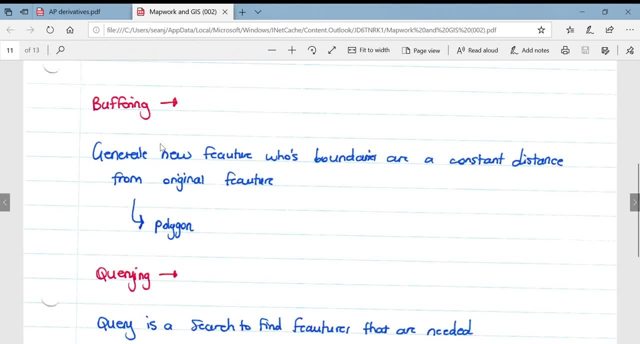 then if we look at data protection, then if we look at data protection, then if we look at data alpha, so these layers are all four working together, but if you want to integrate all of these layers, that you need to create a�, and you will know now. so this was aVESöre, which give you the information about the different. 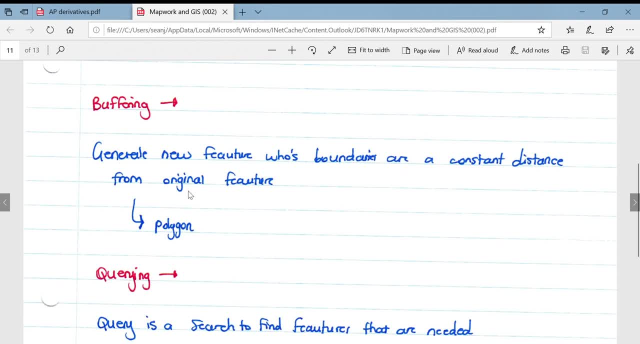 areas and all you'll have to do is go really look into it. so say, for example, here you go, so maybe data羅t, so it's a well-known and you've got a library and system software, but just maybe you want to go out and search for a library. 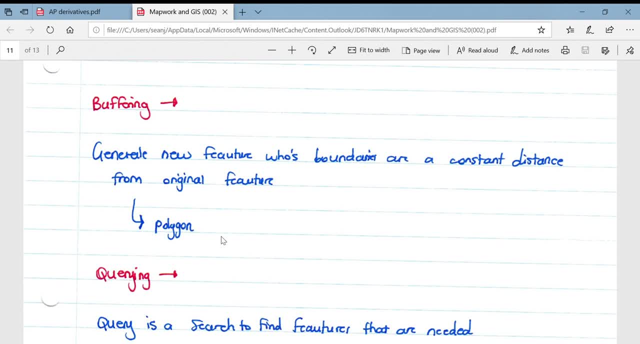 there's also a two kilometer buffer around the limit, around the river, which will indicate the area where there is no, where there's no development allowed in order to protect the river and the surrounding wetlands on the banks of the river. so you would generate this buffer zone and, obviously, you would use your. 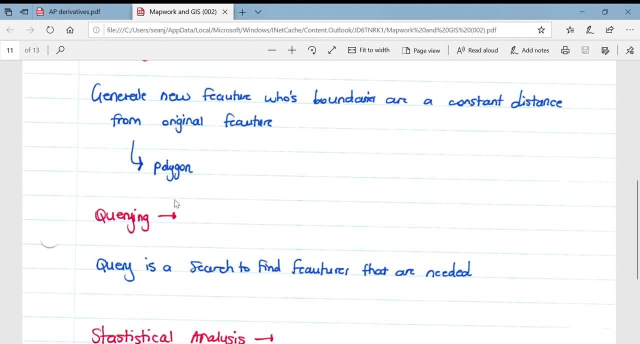 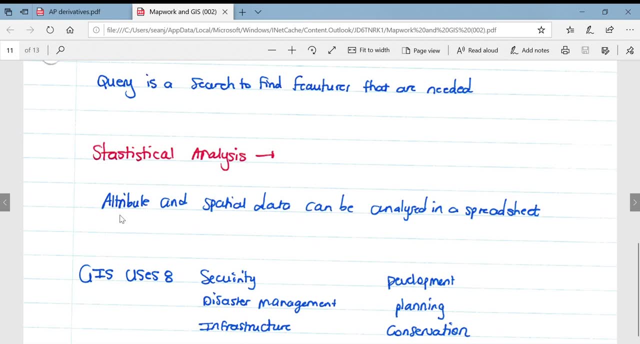 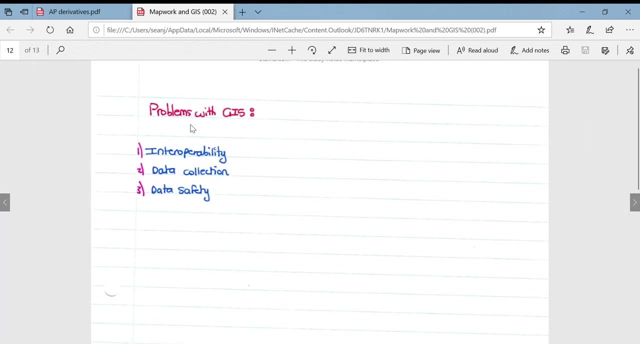 map scale in order to get it into a real life distance- then if we look at querying of data- query is a search to find features that are needed. statistical analysis, attribute and spatial data can be analyzed in a spreadsheet. GIS uses security, disaster management, infrastructure development, planning and conservation- then if we just look at some of the problems with GIS, no need to explain.